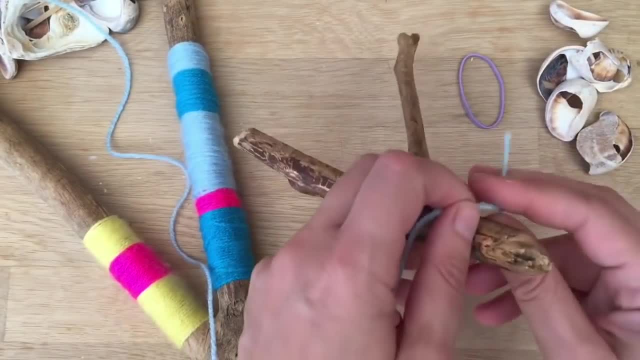 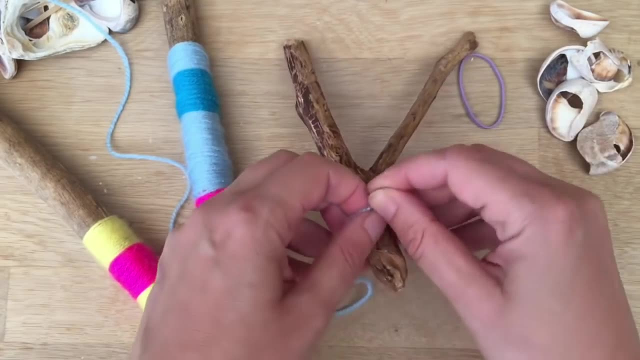 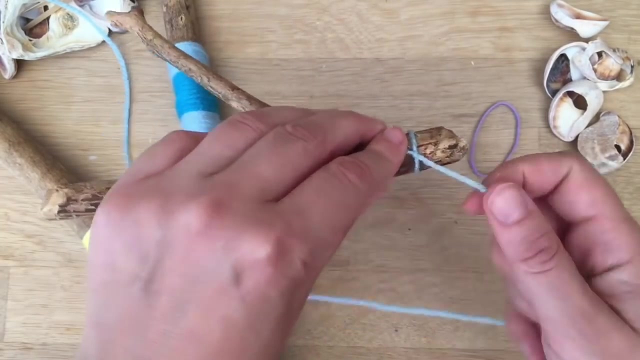 i've got some wool and actually you can do this on the beach too. but you know, it just depends on on what you want to do. wrap it around like this, give it a little knot like so, and then just hold that down, and then you start to wrap like so, now the great thing. 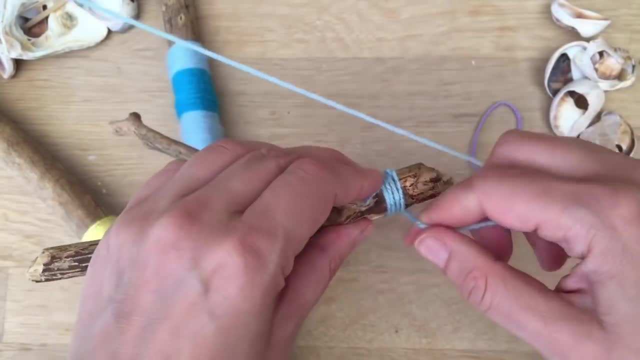 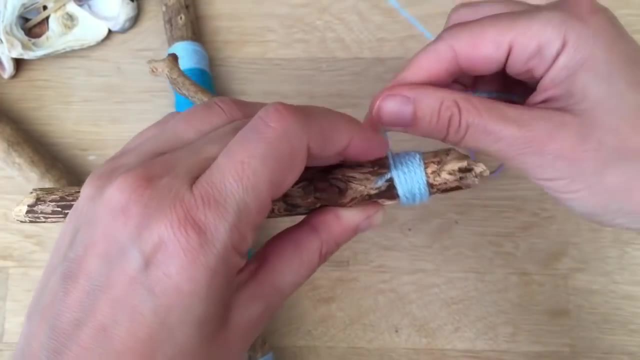 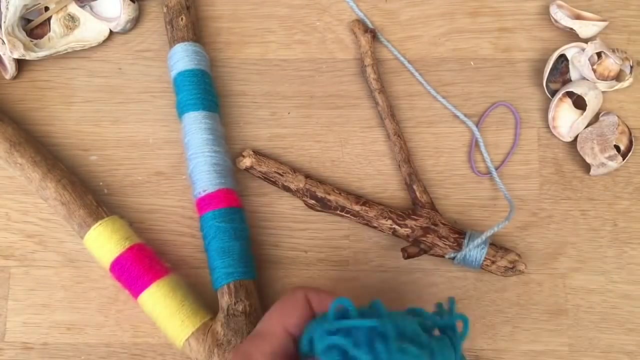 and you try and get that little bit that sticks out covered. if you can see great thing about yarn wrapping, you don't have to be too neat. there we go, that's what you need to do and you keep going. if you want to change colors, all you do is get some more wool, which i have behind me. let's see if i can find an end on this one. 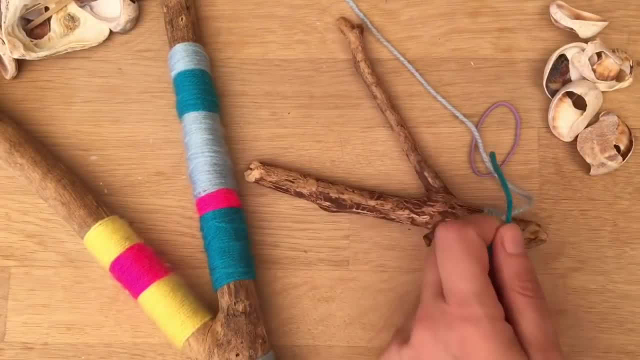 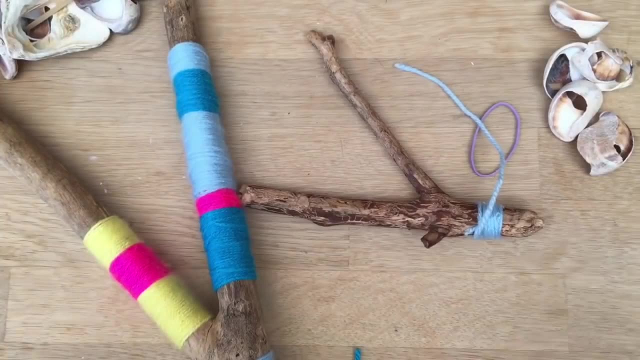 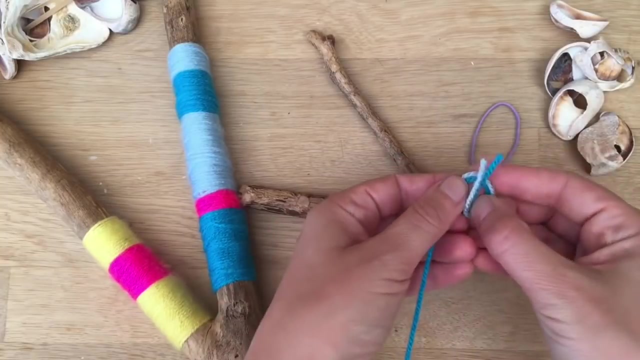 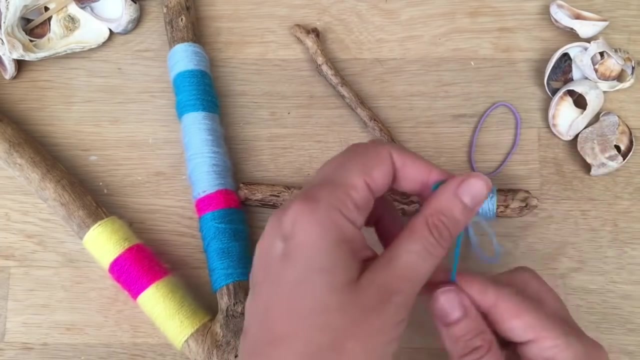 hmm, here's a better end. you get some scissors, you snip it so that one's done. you tie them together by creating a little loop like this, and then you just pull it through, and then you just pull it through, and then you just wrap it around and then you just keep pushing it through. make sure it's nice and tight. 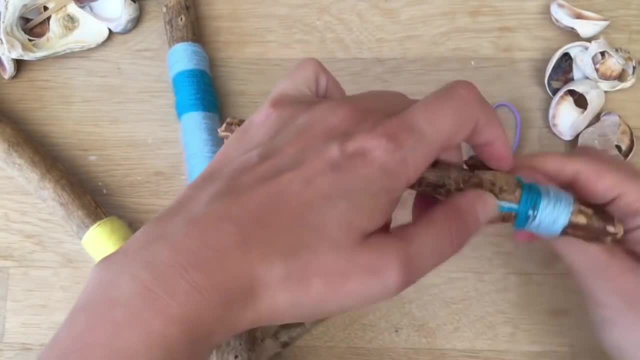 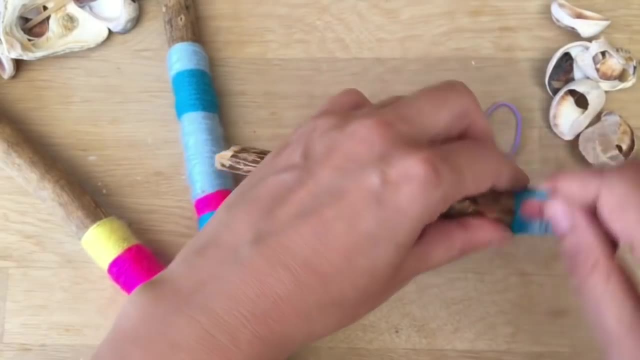 keep wrapping, keep wrapping, and then when you get to the knotty bit, which is, in this case, here again, you hold down the fabric. you know that they're not, so you can cover up some of that, and then every time you sort of go around just gently nudge it down to make it. 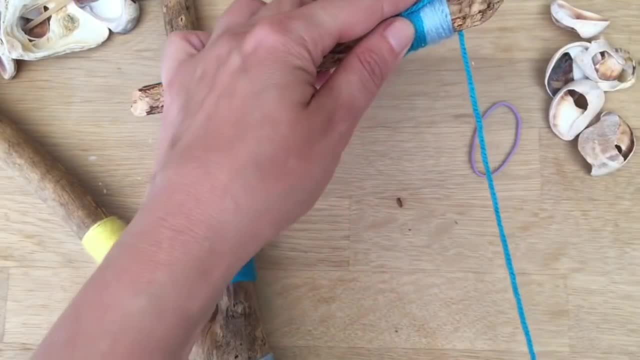 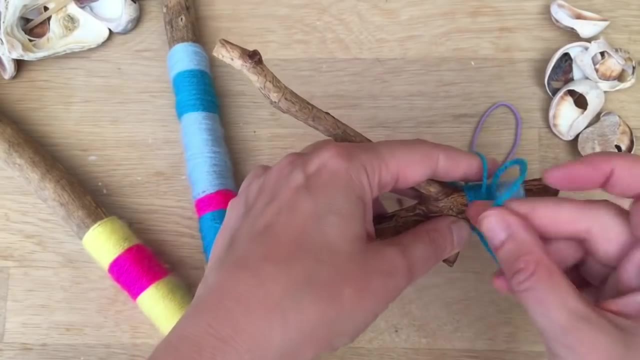 a nice neat wrap. now, when you want to finish off- i'm not going to completely finish this one, because is you take again your scissors, cut it, and then the way i tie it off is i wrap it up, put my finger in in the way and then i thread it through, like so, give it a little tug, do it again. 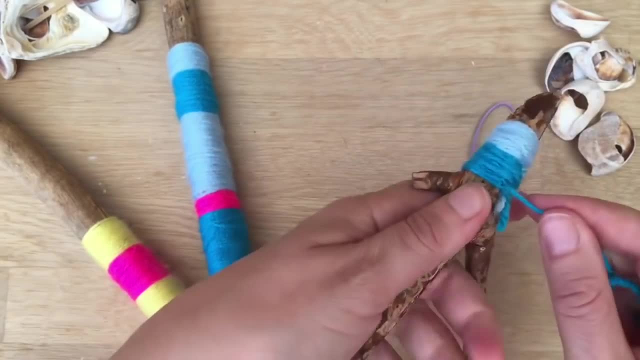 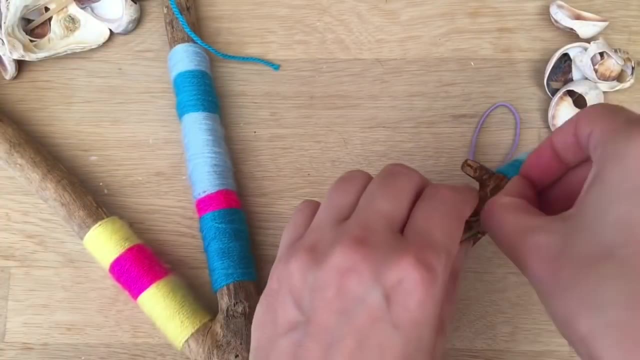 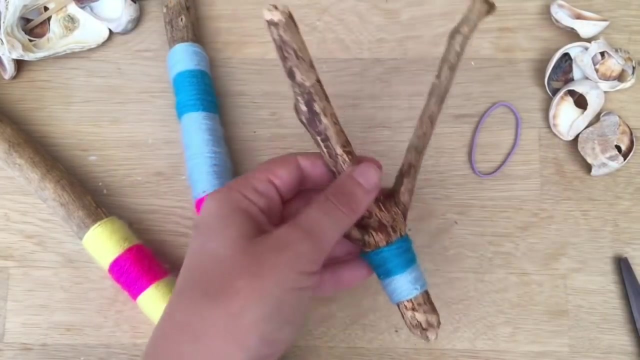 thread it through, give it a little tug, and then, to be honest, and you can trim these things, and i just cut this off and you can poke it inside with something sharp, and there you have how you do your basic yarn: wrapping on sticks. so, and then the fun bit, and 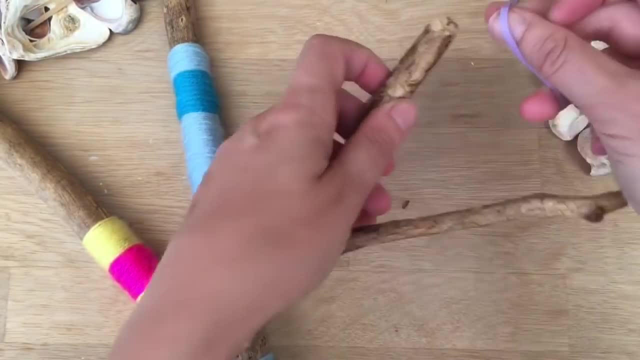 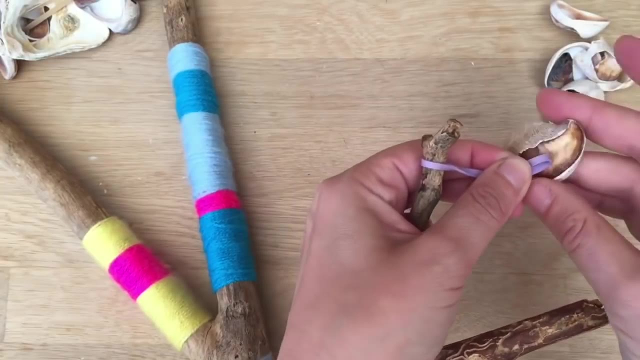 the easy bit. you take your elastic band. of course you can use string, you can use wire, whatever, but i quite like the string method because it's really quick and easy. and then you sort of thread on your shells and it doesn't matter too much in what order you put them. let's get that one next.